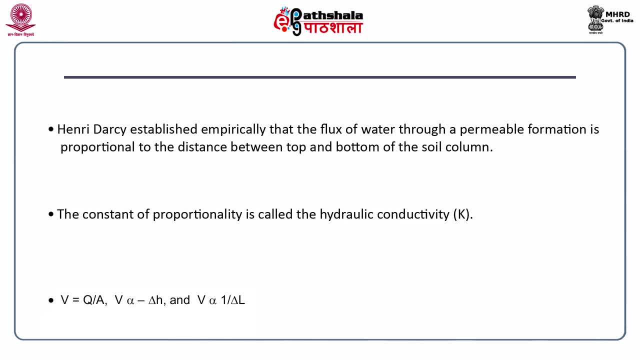 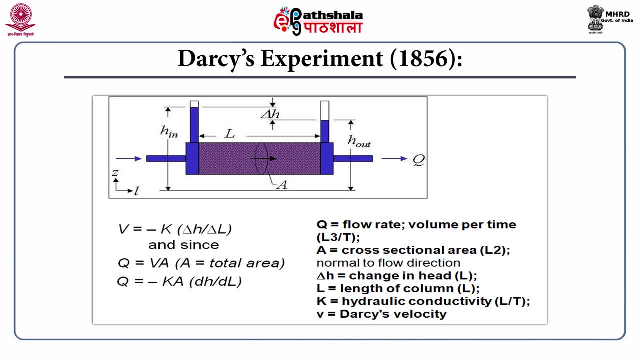 discharge and capital A is the total area of the porous media. This is the picture which shows the Darcy's experiments. So you can see here this is a soil column, horizontal soil column, filled by a porous media having cross section inner, cross section capital. 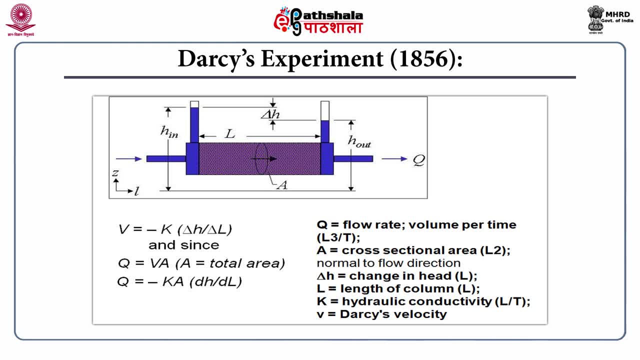 A length of the column is capital L, the head at inlet, that is h in, and the water head at the out plate is the h out. Because the head at inlet is high as compared to the head at outlet, the ground water is going to flow through this column from left to right, producing a 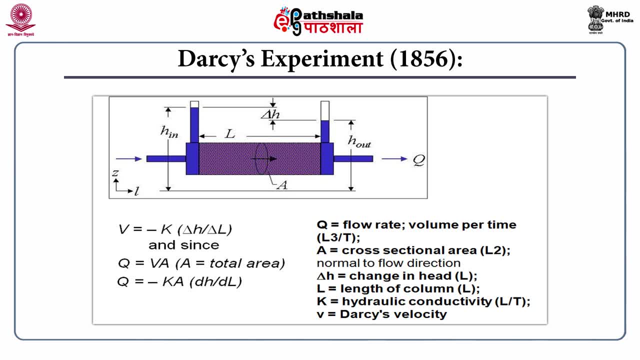 discharge of capital Q. Now, capital Q, which is a flow rate that is nothing but the volume per unit time. capital A is the cross section area of this porous material. delta h is the change in the head head difference, that is the h out minus h in, and capital L is the. 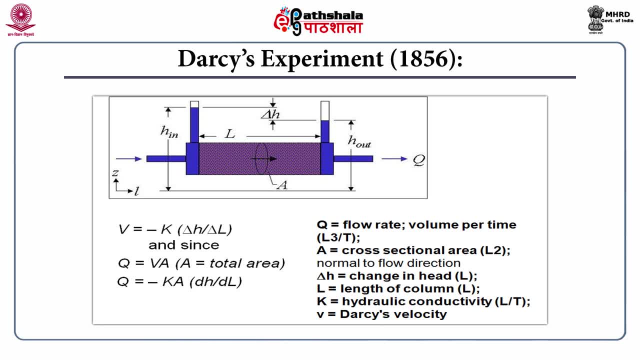 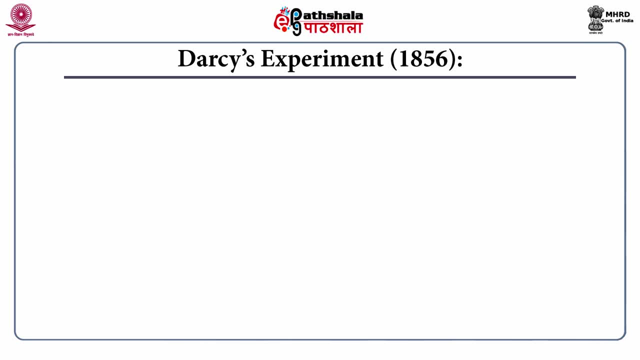 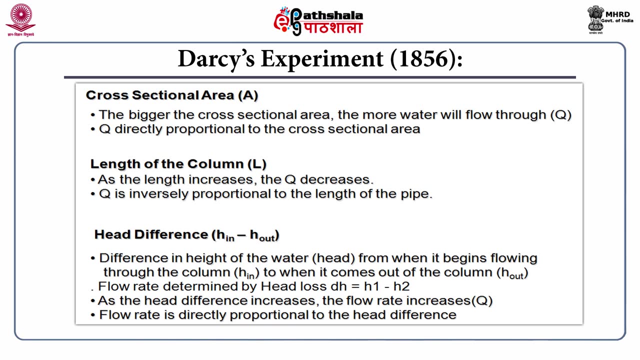 length of the porous media and capital, K is the hydraulic conductivity and V is the Darcy's velocity. So Henry Darcy's law says that when the larger the cross section area, the more water flow through this porous tube. So Q is directly proportional to the cross. 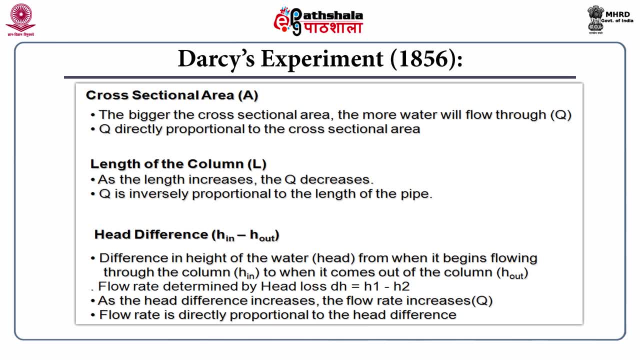 section: area of the porous media length. as the length increases, the Q is going to decrease because when the we increase the length of the porous media, the resistance provided by the porous media is going to be more. So we can just get it. you know the Q is going. 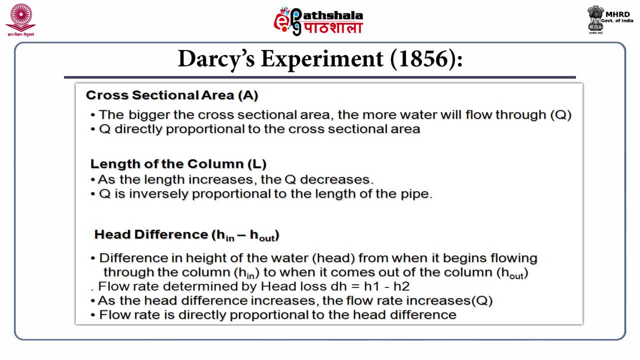 to be less as compared to the lesser length of a porous media, inversely proportional to the length of the pulse media. The last one is the head difference, that is, h in minus h out difference in height of the water, that is head from when it begins. 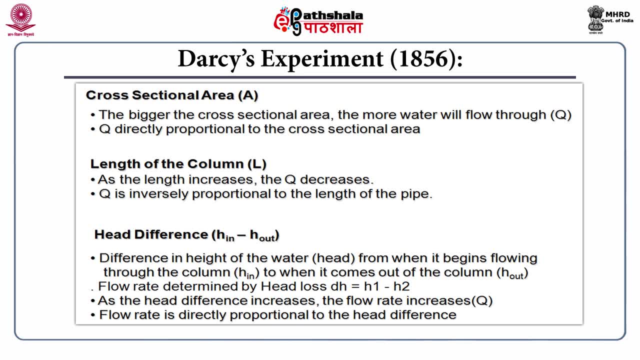 flowing. so the column to when it comes out of the column that is h out. So flow rate is determined by the head loss. as the head difference increases, the flow rate q is going to increases. So flow rate is directly proportional to the head difference. 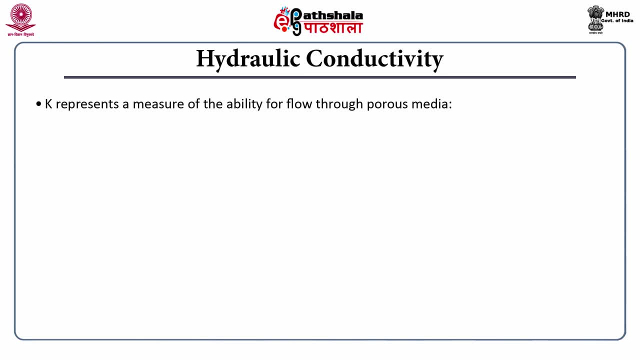 Now the proportionality coefficient k represent a measure of availability to the flow through the pulse media and for the gravels it is value is going to be very high. for the sand also it is very significant, but for the silts and the clay the value of hydraulic conductivity. 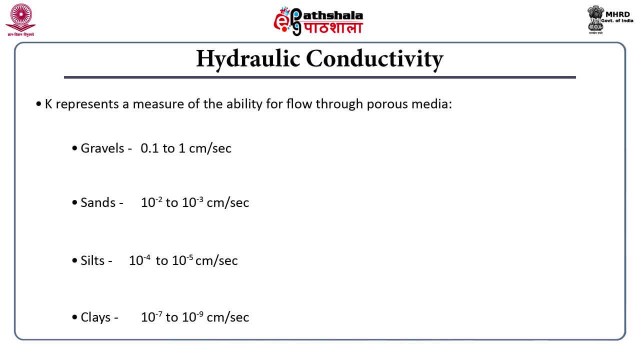 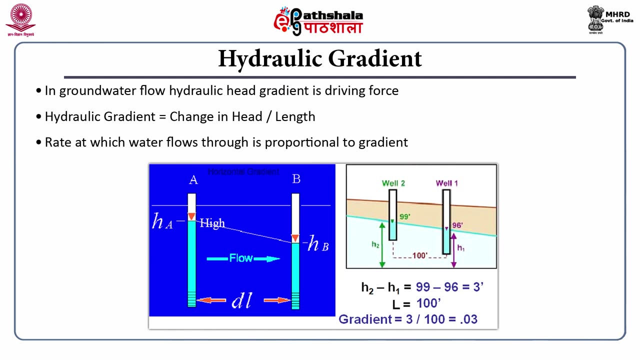 is very less. it means water cannot easily flow through clay and the silt as compared to sand and gravels. Now hydraulic gradient in groundwater flow hydraulics head gradient is the main driving force. Hydraulic gradient is the change in the head divide by the total length. in this picture you can see there are 2 tube wells. tube well. 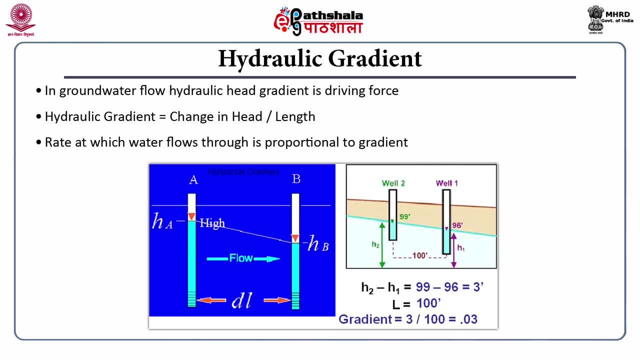 number a and tube well b. the distance between these 2 tube wells is the delta l or d l. the height is h a here and height is h b here. So h a minus h b divide by the distance between 2 tube wells is known as hydraulic gradient, which is denoted by small i. 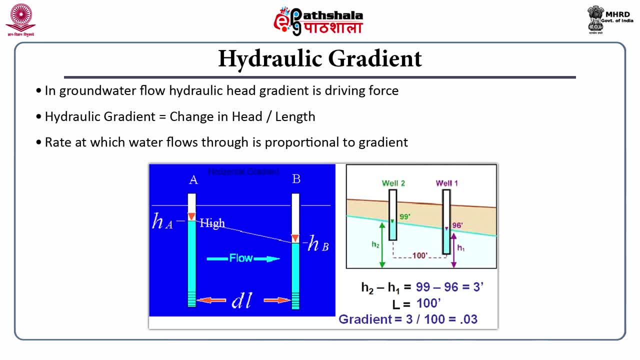 The second picture shows some quantification of this hydraulic gradient: well 1 and well 2.. So 99 feet is the height of the water table at well 2 and 96 is at well number 1.. So groundwater is going to flow from the higher head to the lower head and the distance between 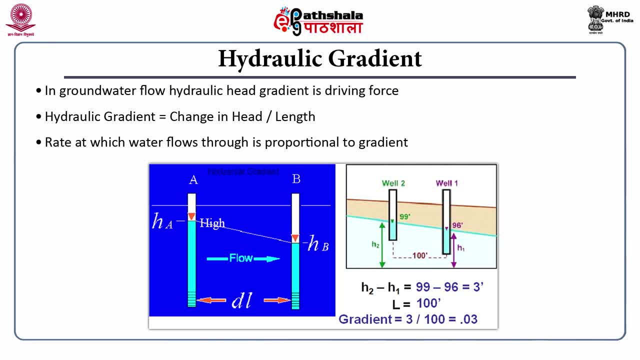 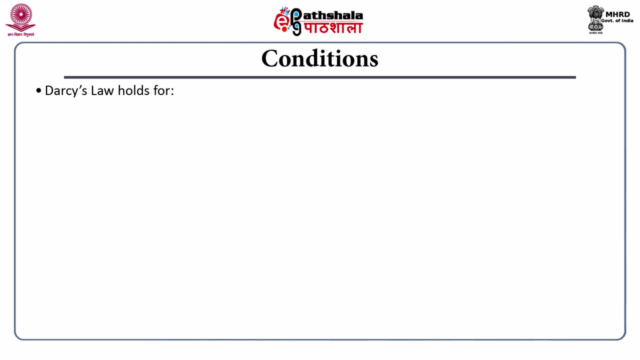 these 2 wells is 100 feet, So we can get. the hydraulic gradient is going to be 99 minus 96, divided by the total distance, that is, 100 feet, we are going to get. i is going to be equal to 0.3 and this is a unit less quantity. Now question come that, where can we can apply. 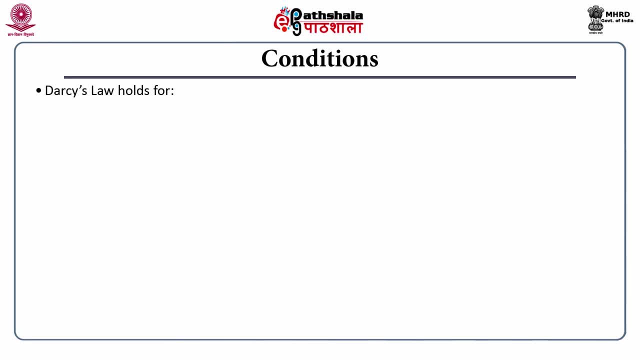 this Darcy's. So Darcy's law is applicable for saturated as well as for the unsaturated flow. A steady state as well as the transient flow type of the conditions can be obtained using this Darcy's equation. Flow in the aqueous acute hearts flow in homogeneous and heterogeneous. 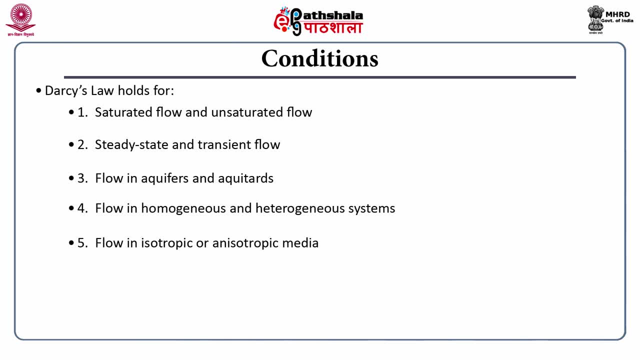 systems can also be obtained using the Darcy's Flow in isotropic and anisotropic media. flow in rocks and the granular media can also be represented by Darcy's law. So Darcy's law apply to flow in any direction, whether it is horizontal or horizontal or horizontal. 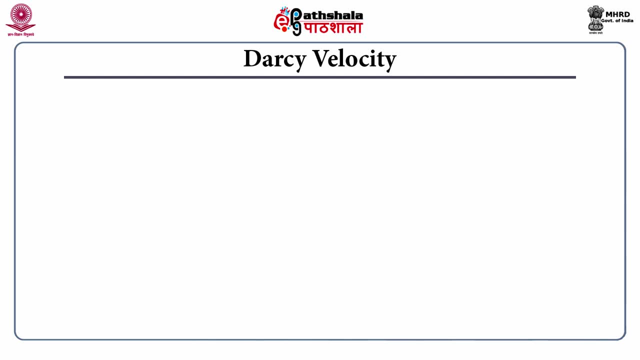 is horizontal, vertical, radial. Now Darcy's velocity, which is denoted here by capital V, sometimes it is denoted by small q, also, So V Darcy's velocity is the specific discharge specifications. discharge means total discharge divided by area, and minus sign indicates that 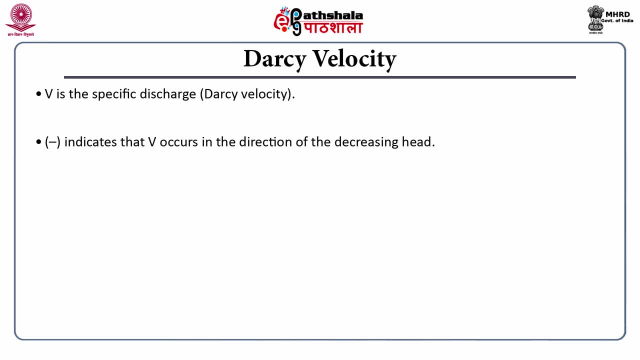 the flow is going to happen in the decreasing head side. Specific discharge has units of the velocity- the specific dishes is a macroscopic concept and is easily measured. The assay velocity is different from the microscopic velocity associated with the actual path And the microscopic velocities are real but are probably impossible or intangible to measure. 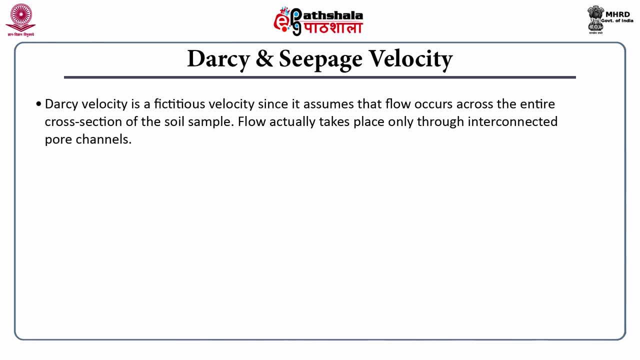 The assay velocity is a fictitious velocity since it assumes that the flow is going to happen across the entire cross section area of the soil sample. The flow actually takes place only through interconnected pores. So you can see here in this picture, this is the section of the porous media where 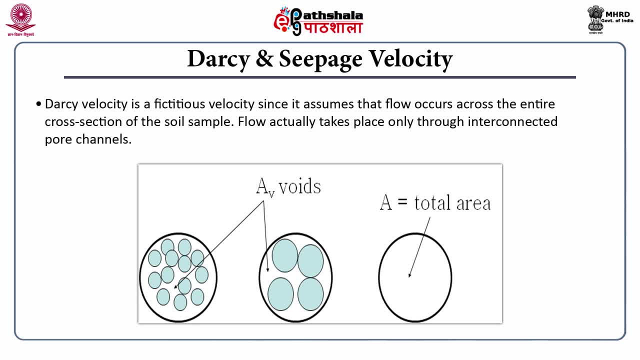 this entire cross section is made of soil solids and soil voids, So when the water is going to flow across this section, it is not going to flow through the entire area A, but the water is going to flow through the openings between the soil. 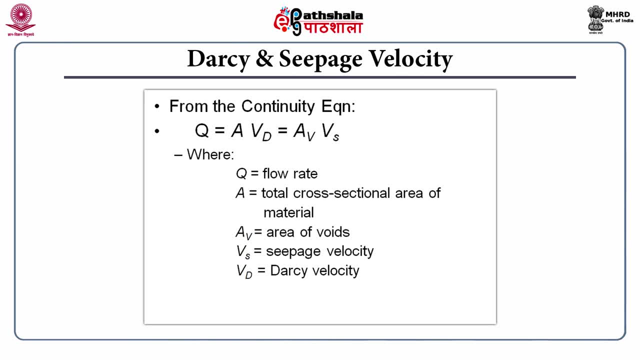 solids And using this continuity equation we can get the relationship between the Darcy's velocity and the actual velocity, The Darcy's. when we divide the Darcy's velocity that is denoted by V D with the porosity, a seepage velocity, V s, can be obtained. 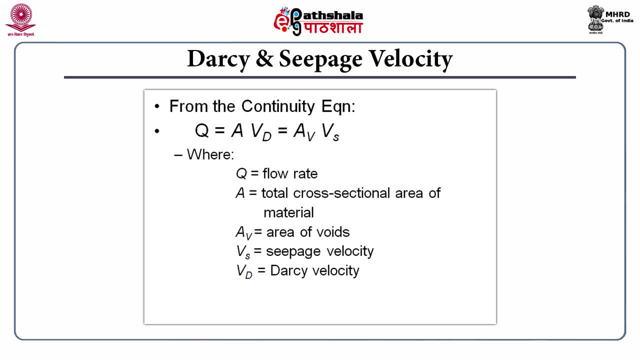 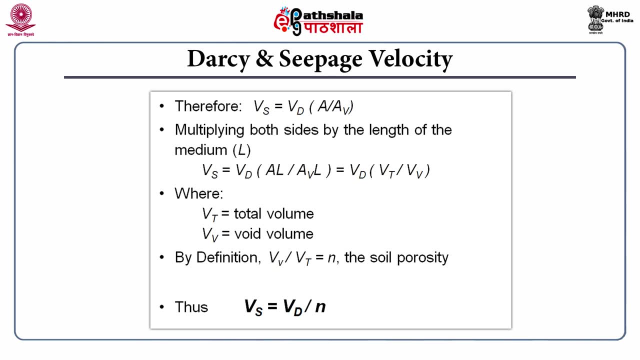 So always the actual velocity or the seepage velocity are going to be much faster than whatever the Darcy's velocity we get from the Darcy's equation. Now the question come that: what are the conditions where we cannot apply this Darcy's approach? 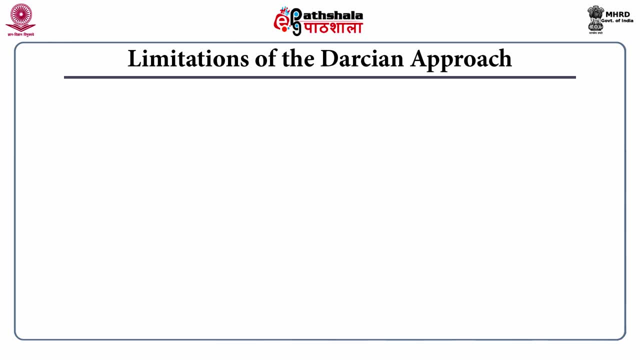 The first is the Day Darcy's law is applicable for the laminar flow. So when the Reynolds number, which represent the laminar Velocity, laminar or the Reynolds, this turbulent type of the flow, So when this Reynolds number becomes very high, it means the flow is going to be turbulent. we cannot get the 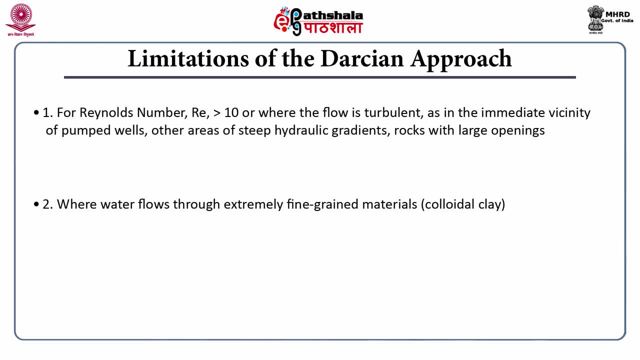 accurate results by applying the Darcy's approach. Second, where the water flow through the extremely fine grained material like colloidal clay, which has the property of shrinking and swelling, we cannot get the appropriate or accurate results from the Darcy's velocity. Under, however, most of the groundwater condition, the velocity is sufficiently low. 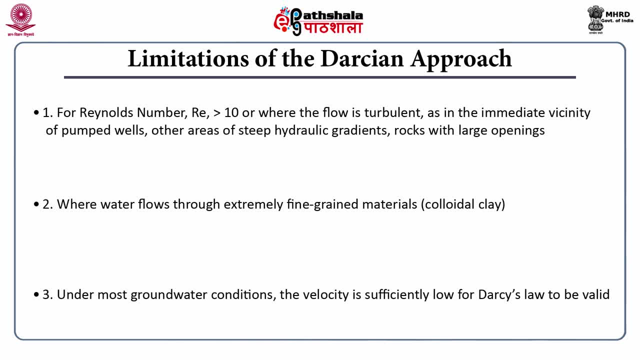 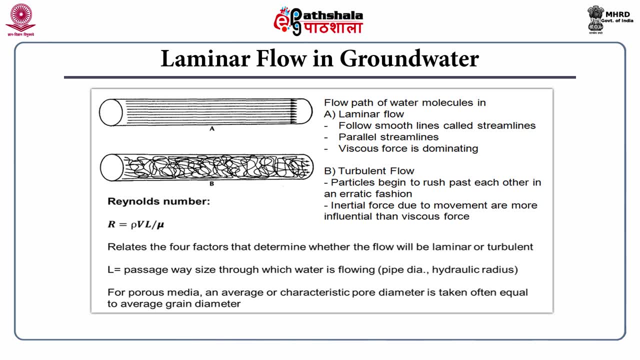 and we can apply the Darcy's law, you know, without any problem. Now this picture shows the laminar and the turbulent flow where the Reynolds number is very small. in the laminar flow, So water particles goes in a stream line parallel to each other. but in turbulent flow the water particles move in a in a random way. 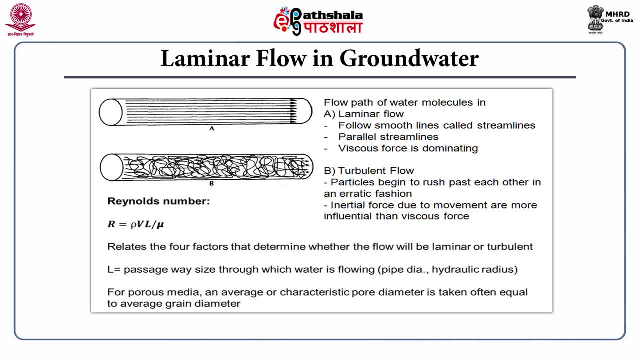 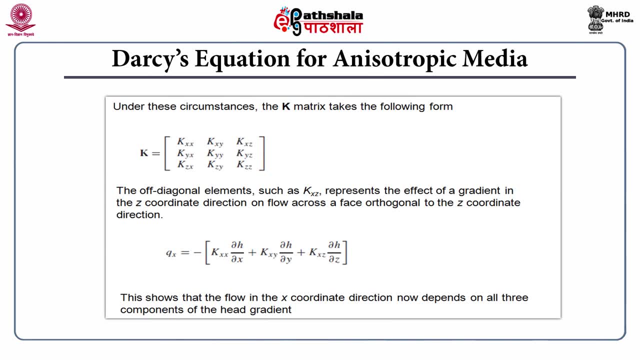 and the mixing takes place significantly as compared to the laminar flow. Now Darcy's equation can be applied in different direction. this is the Darcy's tensor of the hydraulic conductivity capital, K In bold. so this is going to be K x x, K x y and K x g. the second row of this tensor is going to be: 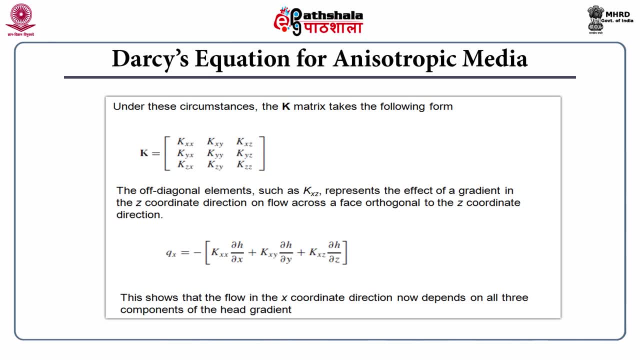 K y x, K y y and K y g. the last row is going to be K g x, K g y and K g g. So K x, K y, K g. so we can. if you want to apply the Darcy's equation in all these 3 direction- x, y and g direction- we can get. 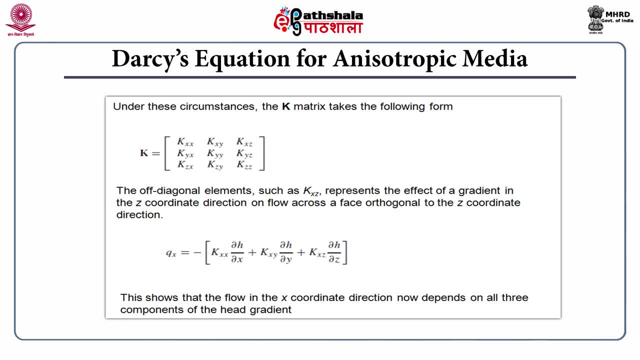 q x equal to K x, d h upon d x. Similarly, for the y direction it is going to be q y equals to K y, d h upon d y. and in for g direction, Q g. the Darcy's velocity is going to be equal to K g, that is, the hydraulic conductivity in g direction multiplied by the hydraulic 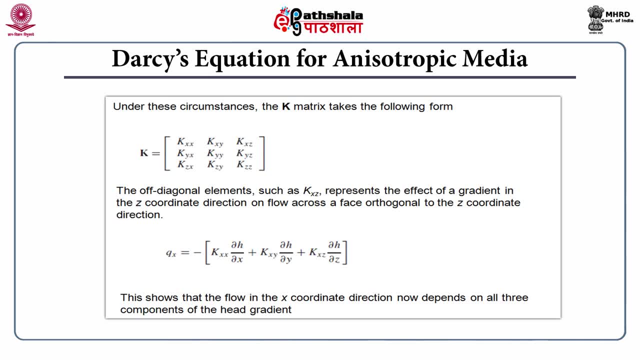 gradient in g direction, that is going to be d h upon d g. This is for the layer type of the phenomena. So if the coordinate axis are going to be oriented with the main direction of this- artisans, you know these directions- then we can reduce this matrix to the. 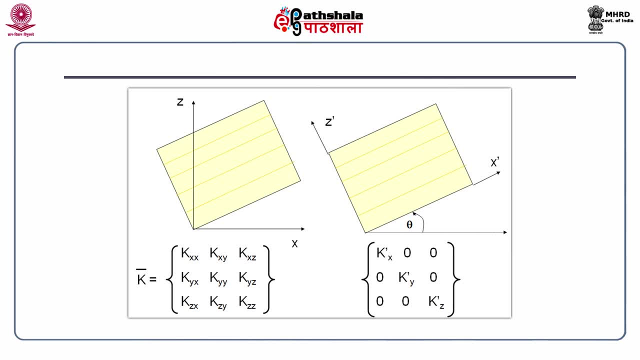 quantities k, x, k y and k g. Now this is the general picture which expands the value of this hydraulic conductivity tensor k in three different directions, having the different, you know, orientation of the of the artisans. you know, coefficient, along with the soil profile. 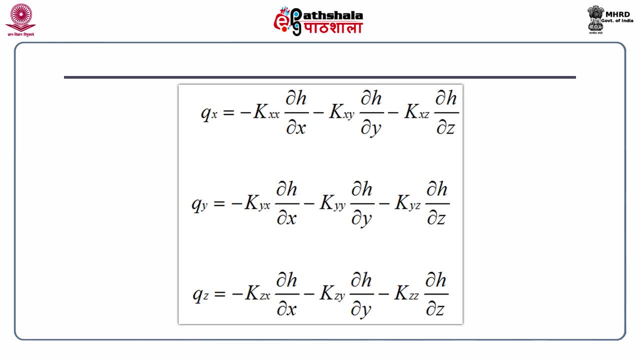 So we can expand this equation, Darcy's equation, for all these three directions, q, x, q, y and k, g. in this manner, And if the main directions are in parallel with the all these x, y and g directions, then we can reduce to the Darcy's velocity to the three main. 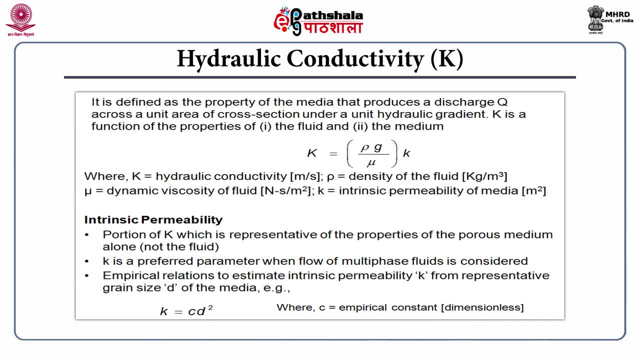 equations. Now, in groundwater hydraulics, hydraulic conductivity is the most sensitive as well as the most important parameters, and that is why the we must, one must you know, quantify the hydraulic conductivity very accurately, So k value that is denoted, denoting the hydraulic 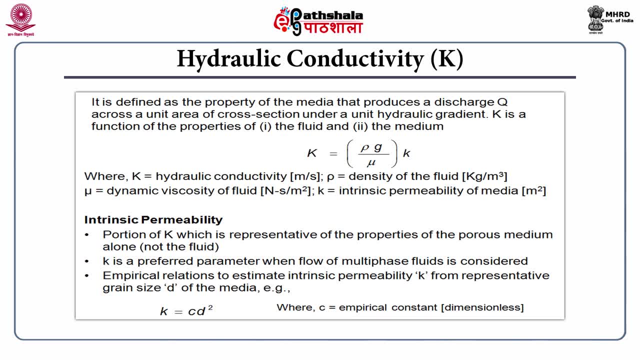 conductivity is comprised the property of the pulse media as well as the property of the fluid. So capital Q is going to be equal to k. So capital Q is equal to rho g upon mu into small k. small k is the intrinsic permeability. 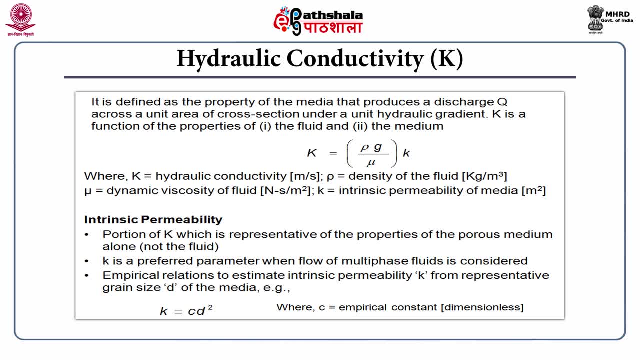 Intrinsic permeability is completely the property of the pulse media and the remaining term, that is, rho g upon mu, are the property of the fluid. So fluid means here we in groundwater. we consider the fluid as a water. So rho g and mu viscosity in draw is going to be. 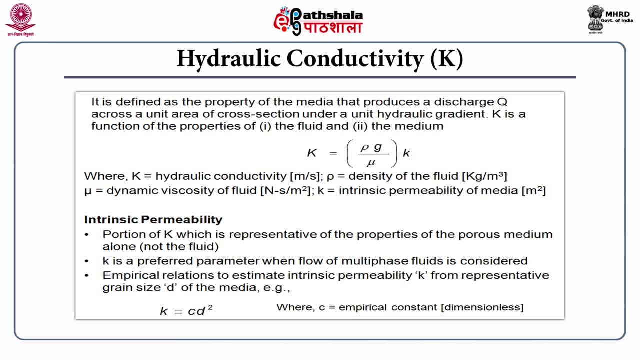 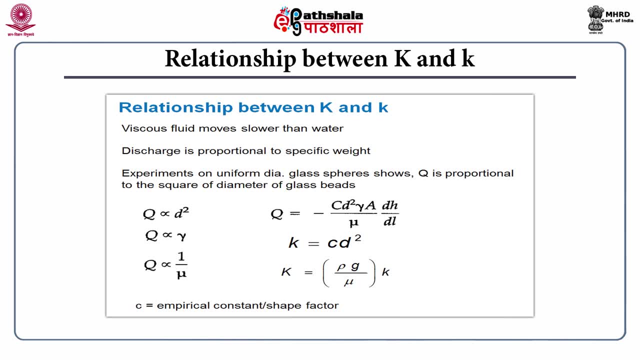 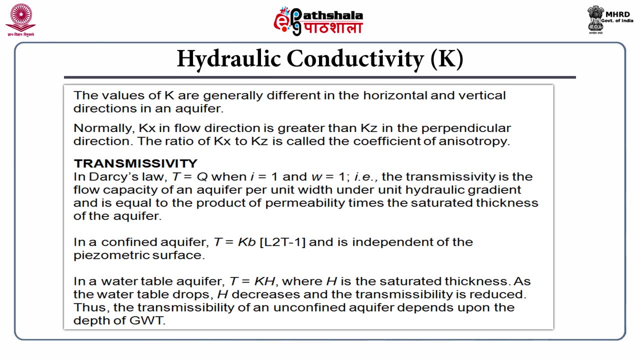 so. So hydraulic conductivity contains the property of the pulse media as well as the, as well as the fluid passing through this pulse media, And this is the relationship between this intrinsic permeability and the hydraulic conductivity capital K. We can use the hydraulic conductivity for getting that formation coefficient in. 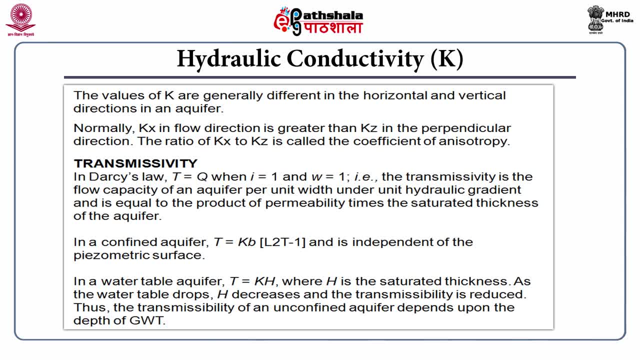 form of the transmissivity of aquifer. Hydraulic conductivity is a is a property of the porous media which is showing its how easily water can flow at a point location. When we talk about the entire capacity of the aquifer, then if you this multiply the hydraulic conductivity. 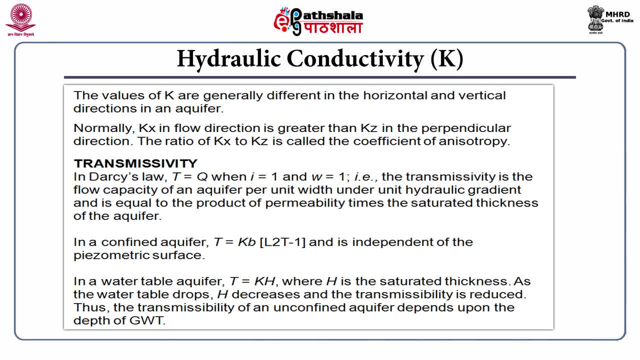 with the total water. So this is the relationship between the intrinsic permeability and the total thickness of the aquifer. we obtain the transmissivity. Transmissivity or transmissibility are the same thing. So K into B is nothing but the. 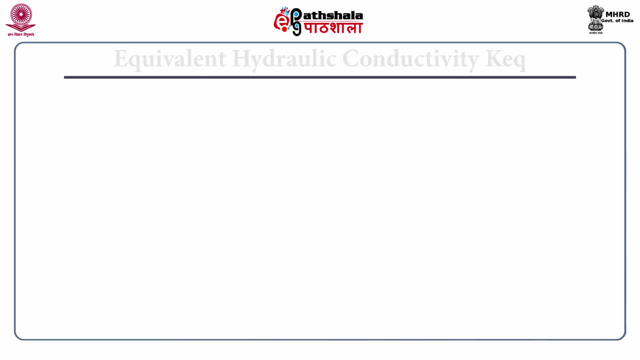 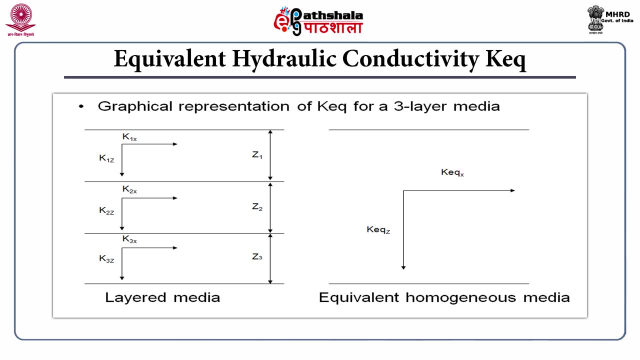 capital T, that is known as transmissibility. Now, sometimes the aquifer media is not going to be homogeneous. it can be stratigraphic or it can going to be different types of the layers, So in that case it is important to get the equivalent hydraulic conductivity. 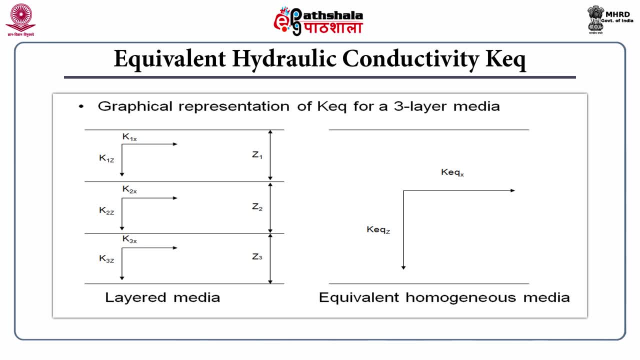 So this picture shows that there are 3 different layers of the porous media having thickness G 1, G 2, G 3, having different hydraulic conductivity in x and g directions. So for getting the equivalent hydraulic conductivity, that is, in x direction as well as in the vertical. 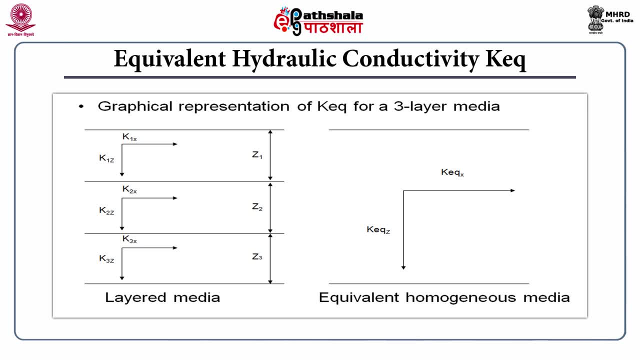 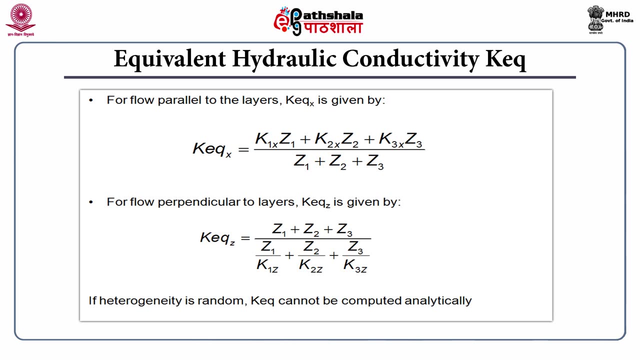 direction, in g direction. we can use this equations for getting this equivalent hydraulic conductivity across the flow as well as parallel to the. this clay layers, soil layers. Similarly, transmissivity can be obtained by taking the average. it is the summation of the different T 1,, T 2,, T 3,, T 4,, T 5,, T 6,, T 7,, T 8,, T 9,, T 10,, T 11,, T 12,, T 12,, T 12,, T 13,, T 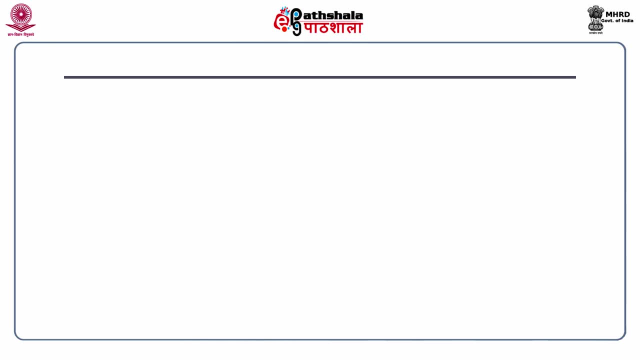 such type of the formations. Now there are different methods for obtaining the hydraulic conductivity: empirical methods, based on the correlation of the grain sizes with the, and the second one, the laboratory method, using the directly this aquifer material putting into the equipment that is known as. 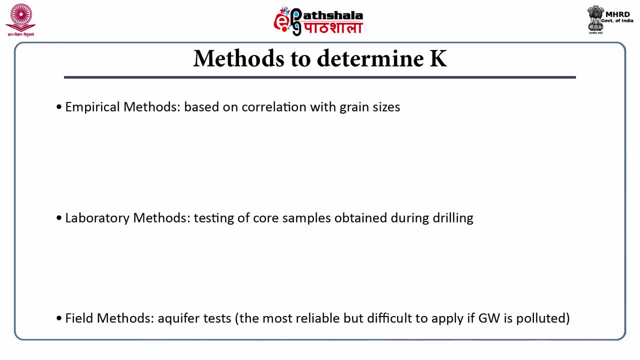 permeameters. and the last one is the field methods. aquifer test are generally performed for getting the aquifer parameters, especially hydraulic conductivity, storage copiators. Now, let us go to the next slide. Now, let us go to the next slide. Now, let us go to the next slide. 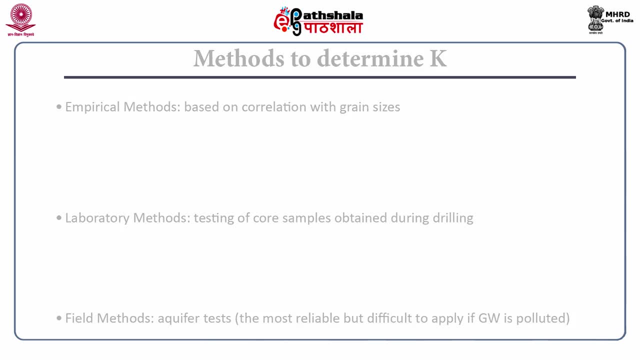 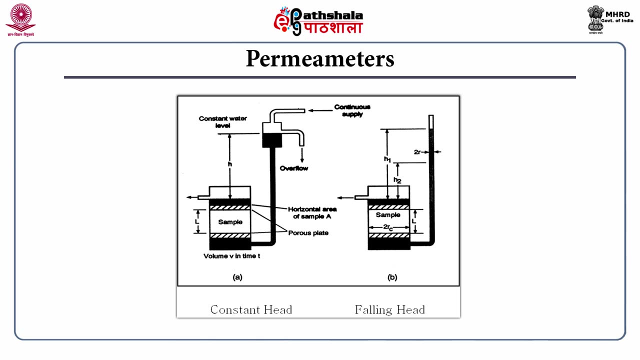 So we are going to discuss the permeameters. which is coefficient and transmissivity? we are going to discuss them. So this is the permeameter which is generally used for measuring this hydraulic conductivity. here you can see this is the sample of the aquifer material which is put here in this. 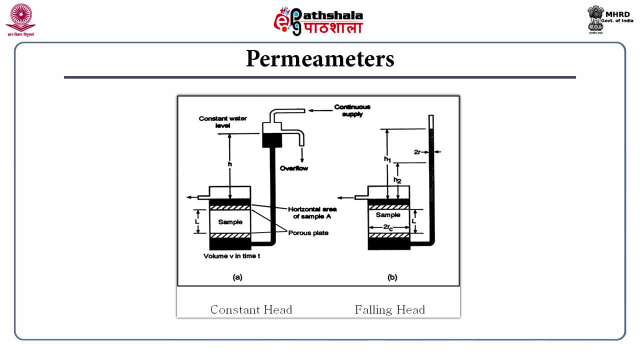 apparatus. there are 2 types of the permeameter: the falling head as well as the constant head type of the parameters used. when the grain size of the aquifer material is quite coarse, the falling- the constant head type of the permeameter is used. but when the particle 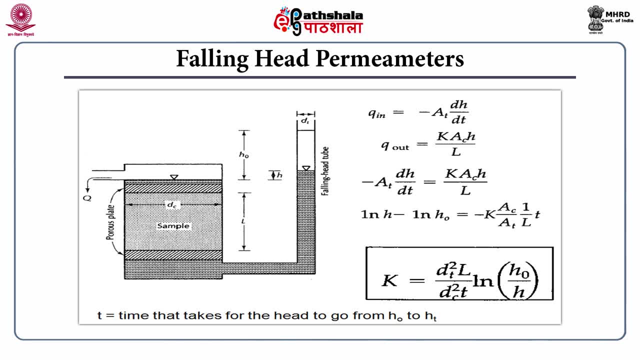 size is very small. in that case, the falling head permeameter are useful for getting the hydraulic conductivity value of the aquifer material And these are the equation which can be used for getting the hydraulic conductivity from this falling head as well as from the constant head type of the permeameters. 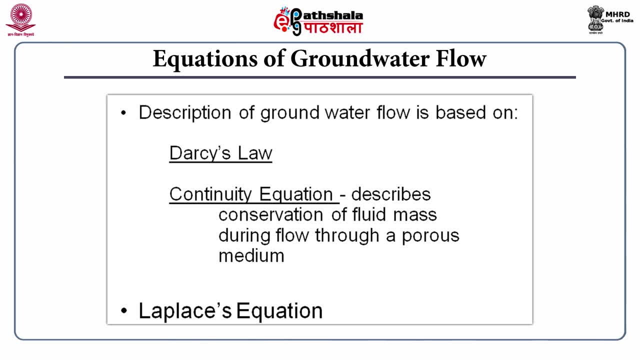 Now for deriving the groundwater flow equation. we are going to use Darcy's equation, that is, q equal to k, ai, and the second is going to be continuity equation- continuity equation mean nothing- the mass balance equation. So by integrating the Darcy's law with the mass balance equation, we are 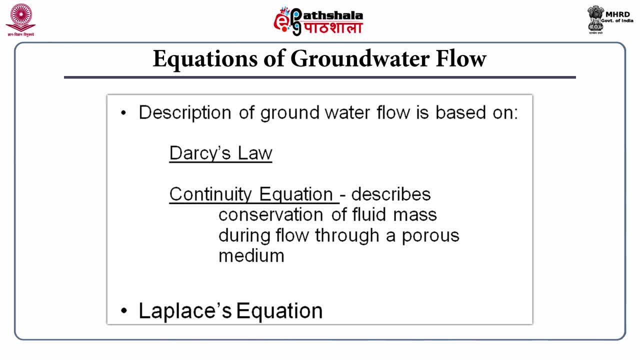 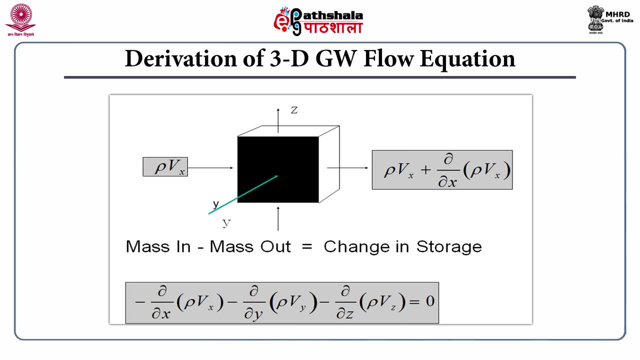 going to obtain the groundwater flow equation, and the specific form of the groundwater flow equation is known as Laplace equation. So this is the picture which shows a parallelogram having a dimension of x, y and g. You can see here there are total 6 faces of these cuboids. 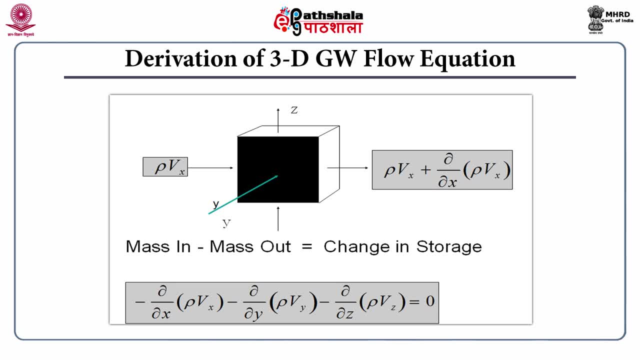 from, let us consider from 3 faces the water is entering and from the remaining 3 faces water is leaving to the system. So by considering the x, y and g direction, we consider the flux in the x direction. So that is the v x, that is, this is the Darcy's flux: v, x and the change in 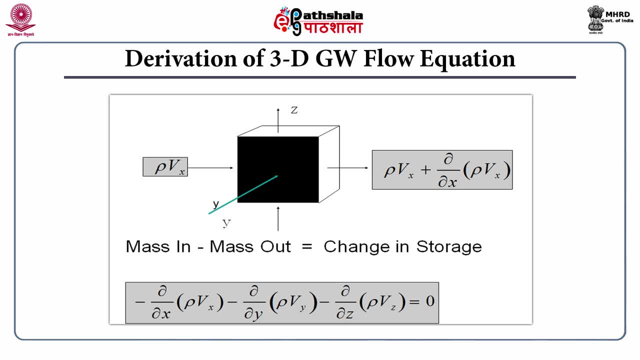 this direction. flux is going to be v x plus d upon dx into v x and by considering the mass in minus mass out, that is going to be equal to change in storage, because change in storage is going to be completely saturated zone. So we can say the change in storage is going to be: 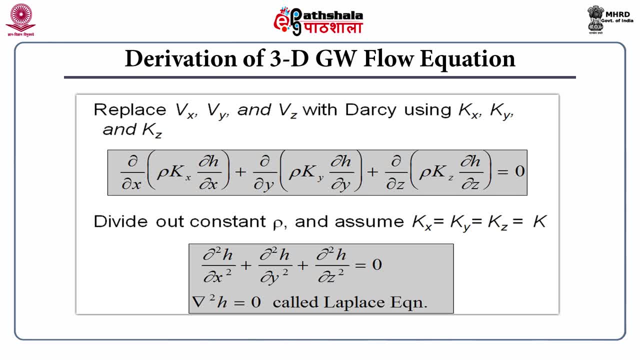 0 is 0. Theta is going to be theta s. So by putting all these 3 direction values we can get this equation d upon dx into v, x, d upon dy, into vy, d upon d, g to v, g equal to 0.. Now this v, x, v, y and v. 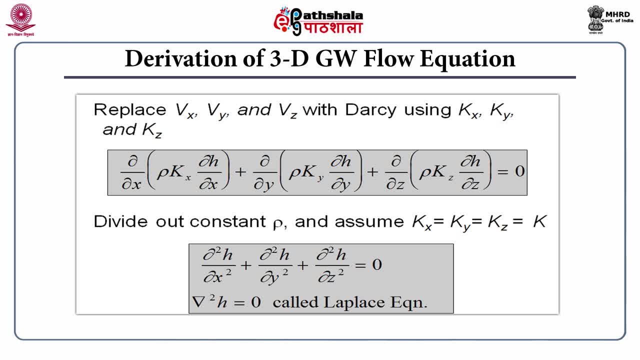 g are nothing but the Darcy's velocity in x, y and g direction. by replacing these Darcy's velocity from the Darcy's law, we can obtain this equation here, and this is the general ground water flow equation, while considering no change in the storage. 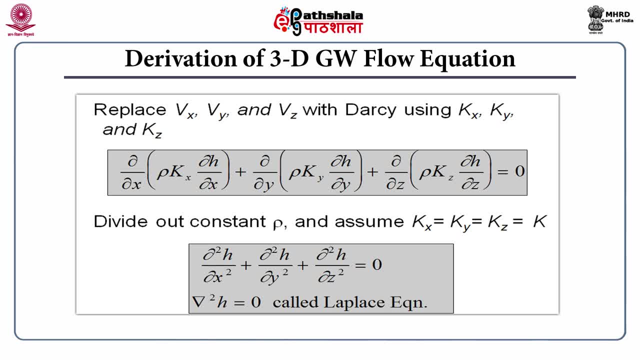 Now if you consider a k, x equal to k y means completely homogeneous and isotropic type of the aquifer material, then this k, x, k, y, k, g equal to be can be taken out from this equation and this will become 0 and the resulting in: we are going to get d 2 h upon dx square plus d 2 h upon. 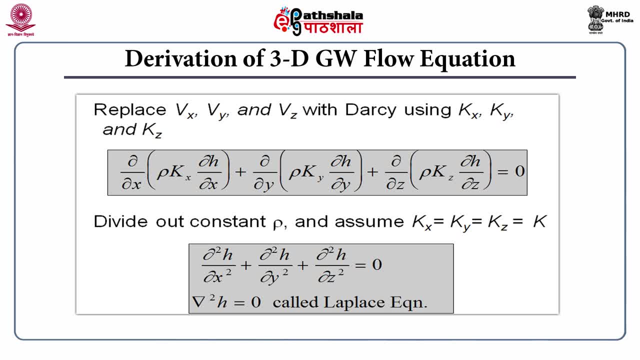 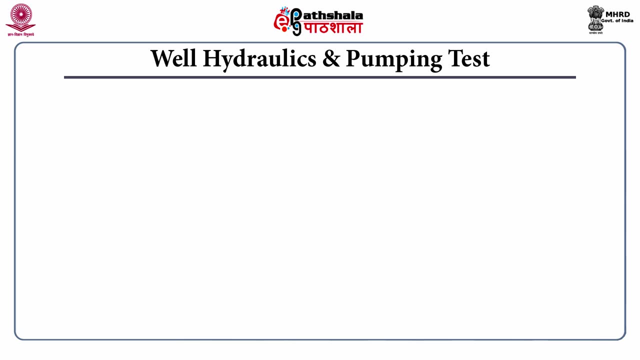 dy square plus d 2 h upon d g square equals to 0, and this is known as famous Laplace equation. Therefore, quantifying homogeneous and steady state groundwater flow in in sub-surface. Now, well, hydraulics is very important. it is not on. the wells are not only the source of the 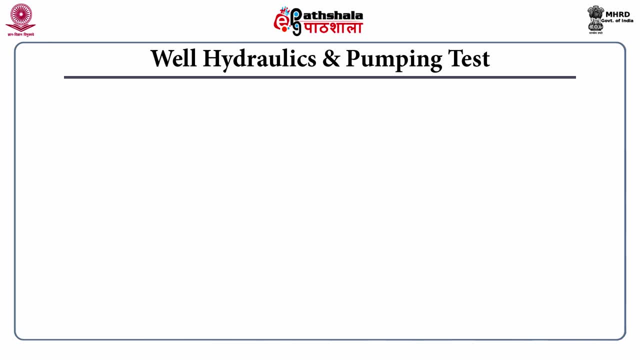 exploring the groundwater, but they are also used for characterizing the aquifer aquifer parameters. So generally pumping tests are done in the field for getting the aquifer parameters. So the principle of pumping test involves the applying the stress on any aquifer by 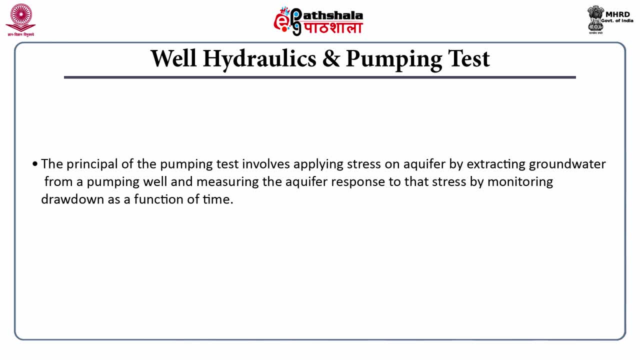 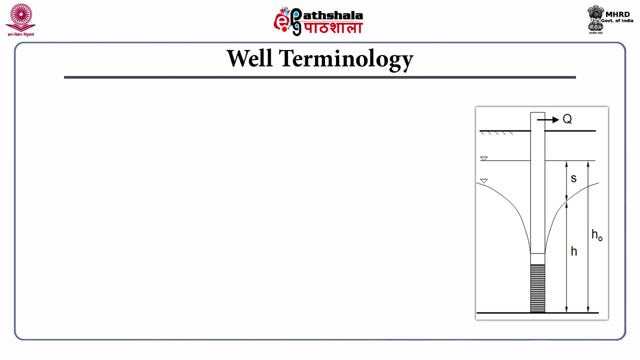 by extracting the ground water from the pumping well and measuring the aquifer response to that stress by monitoring drawdown as a function of time. So this is the typical diagram which shows the a hydraulic well and these are the different terminology which are associated with the well: hydraulics. 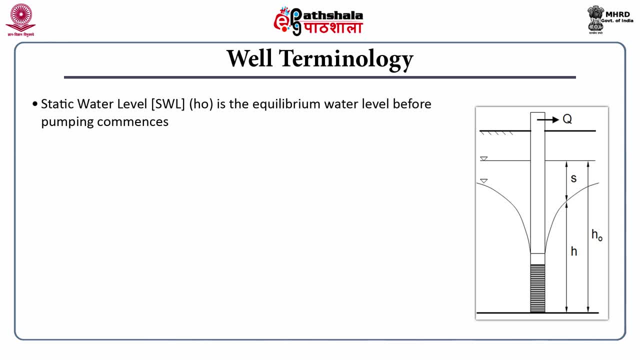 The first one is the static water level, that is, SWL. this is the water level before pumping is started. then pumping water level- PWL is the water level during the pumping and the drawdown is nothing but the difference between the pumping water level and static water level. 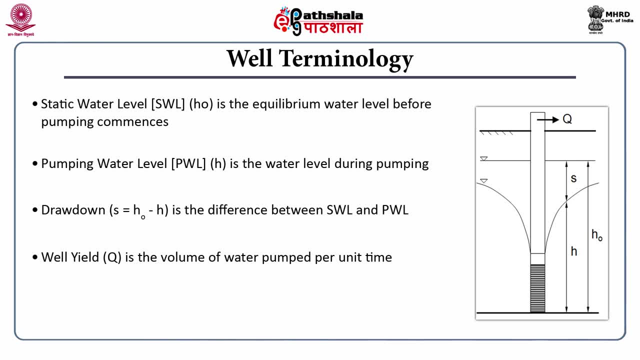 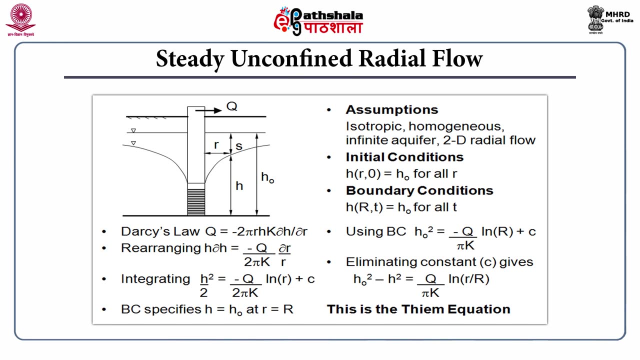 denoted by small s well yield is the volume of water pumped per unit time, and then specific capacity. if you will divide the pump yield with the resulting drawdown, we get a specific capacity. Now for steady state, Unconfined radial flow. we can consider a well fully penetrating in an unconfined aquifer. 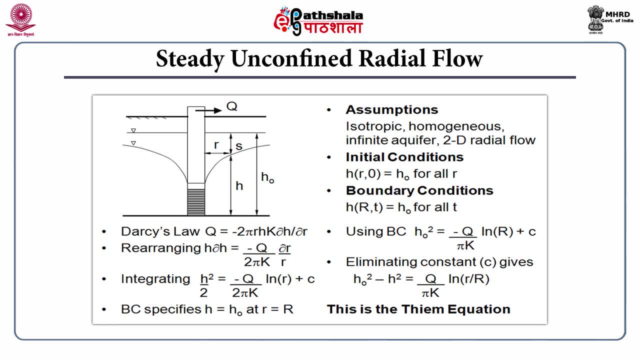 by considering that it is a completely isotropic, homogeneous type of the aquifer media. Now, by applying the Darcy's equation: because q is constant here, so we can say q equal to ki, so capital Q is going to be equal to k. that is hydraulic conductivity of the aquifer. 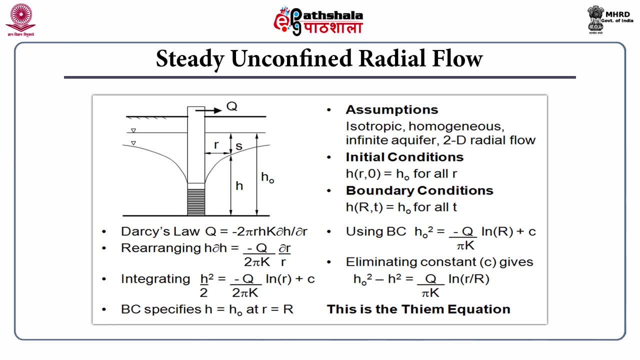 in which this hydraulic well is drilled. By using this hydraulic gradient, we can say that h will be equal to 1 pi R by 2 pi r A into Dnieper's gradient, into area. this area is the water which is contributing to the 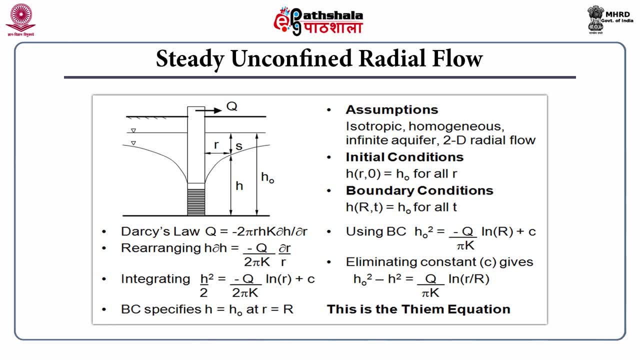 annular region of this. well, So this is going to be hollow cylinder of r distance. let us say so. 2 pi r is the perimeter and the h is the total thickness of this cylinder, So we will get that total area. 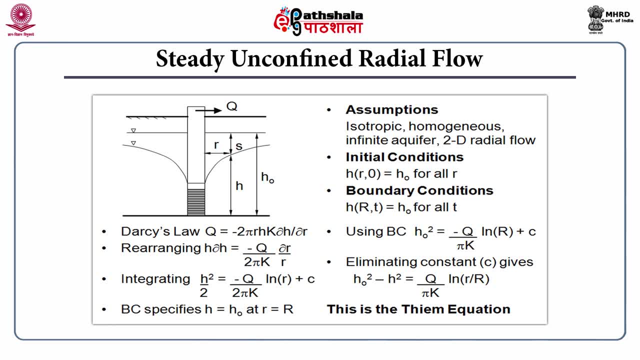 d r, So q equal to 2 pi r into s, that is area, into k hydraulic conductivity, into hydraulic gradient, that is d h upon d? r. By rearranging we can get d h into d h is going to be minus q upon 2 pi k- into d r upon d? r and by integrating this equation with respect to h we can get 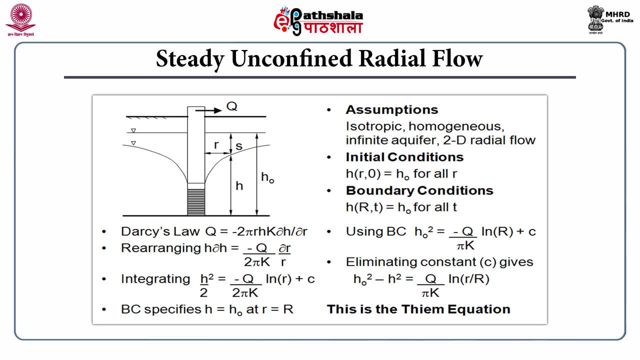 h square by 2, equal to q upon 2 pi, k, ln plus integration coefficient c, And by applying the boundary conditions, h equal to h naught. it means at radius of influence, where there is no drawdown, we can put small r is going to be capital R and we can obtain the value of. 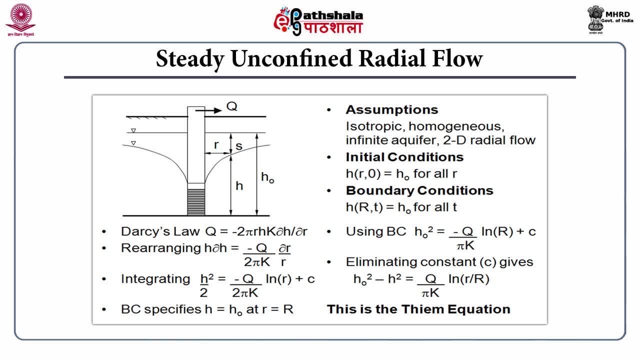 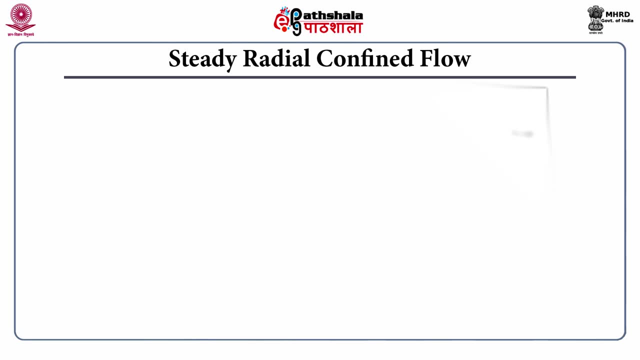 capital C and can find out the popular Themm's equation representing the water table profile at any pumping time. So h naught square minus h square equal to q upon k, pi k into ln, r upon capital R. Similarly we can obtain the radial: 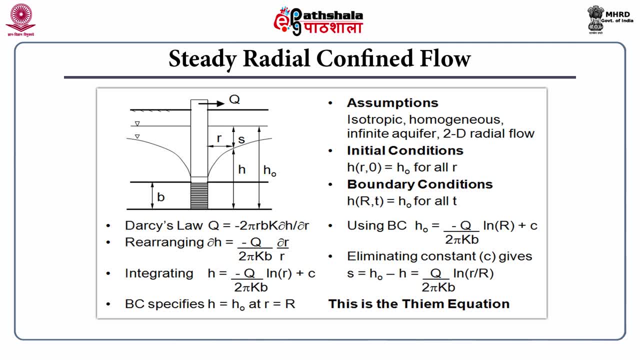 flow in a confined aquifer having a thickness of small v, we can apply the Darcy's equation. The only difference here is the total area. in earlier case it was 2 pi? r into s that, the entire area which was contributing, but here, because the thickness of the confined aquifer is small b. 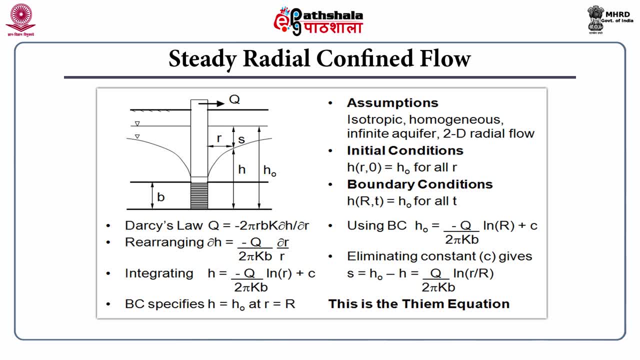 So the total area which is contributing to this water flow in this well screen is going to be 2 pi r into b, k, d, h upon d r and again by rearranging and by applying the boundary conditions, we can get this equation representing the drawdown small s equal. 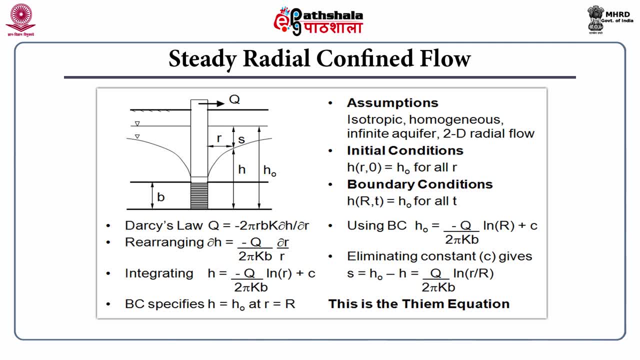 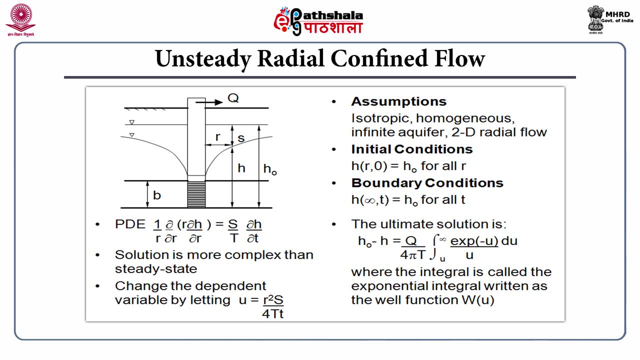 to h naught minus h. this is the difference between the pumping water level and the static water level is going to be equal to q upon 2, pi, k, b, ln, r upon capital R. Now for conducting the pump test. for each flow types, we need to detect the left and right flow stroke in the tank. So there is a very big difference. So if we take a look at the flow type speed, So if we take a look at the flow type speed, then we will be able to find this equilibrium condition or steady state condition, or the ideal type of the flow approach For characterizing the aquifer. parameters are very important things, so we will may have to find out how much the flow is going to be. In such a case we generally do this field test for finding out the aquifer parameter and characterization of the different, any other formation coefficients. Finding this equilibrium condition or steady state condition is very time taking and also one has to extract a load of groundwater at the surface. So in that case we can go for an unsteady radial type of the flow approach for characterizing the aquifer parameters. 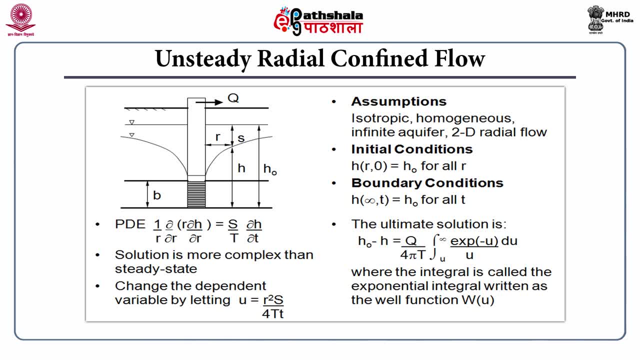 This is a partial differential equation which can be solved for getting the aquifer parameter value s and t from confined and unconfined aquifers. So here small u represent this. this is the auxiliary function. having r square s upon 4 t into t, r square is the r is the radial. 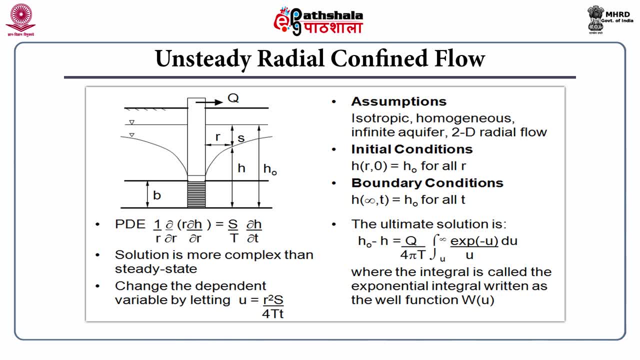 distance, capital S, this storage coefficient of the aquifer, and capital T is the transmissivity and small t is the time of pumping. and the solution is given here: that S, that is nothing but H naught minus h, is going to be equal to q upon 4 pi t integration, e to the power minus u. 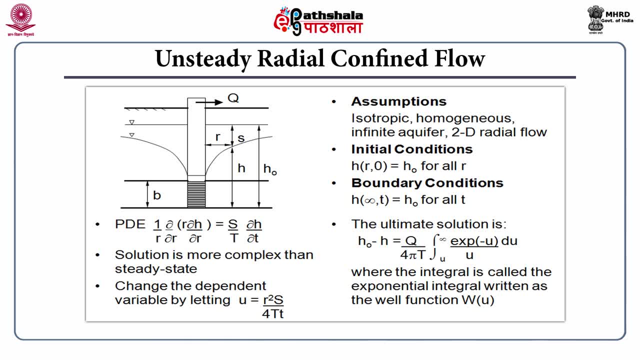 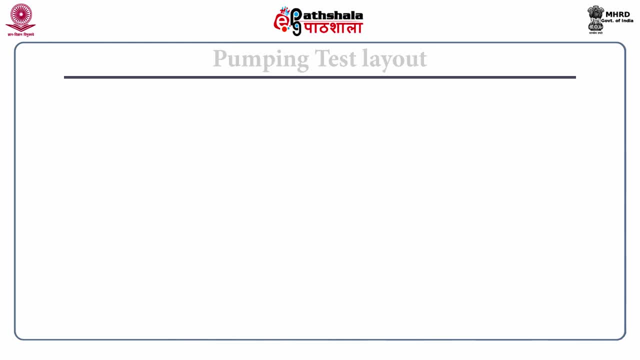 upon u into dot u. So this is the well function. this entire integration quantity can be termed as a well function w? u. Now, using this auxiliary function and the well function, we can plan a pumping test in the field. So this picture shows the 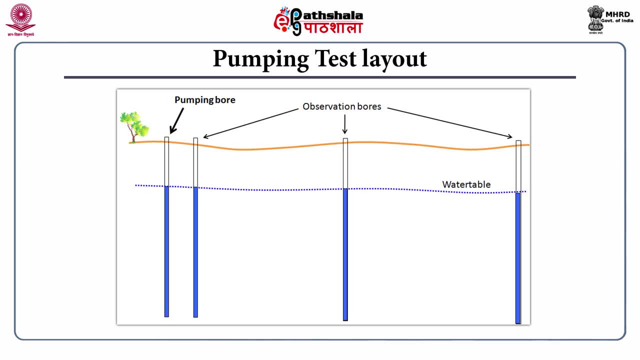 pumping test in the field. So this picture shows the pumping test in the field. So this picture shows the pumping test layout. this is the ground surface and we are having a pumping well denoted by this solid arrow, and then nearby to this pumping well. 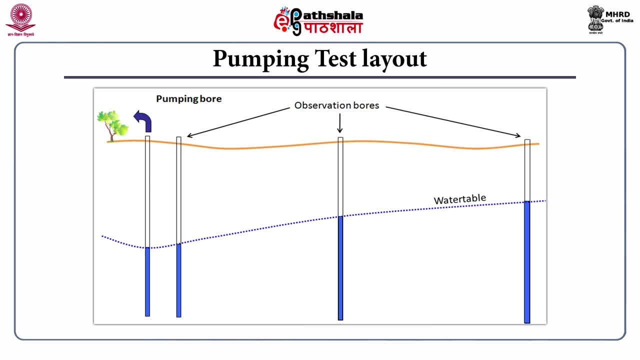 there are three observation wells. Now when the pumping starts from this main pumping well, the water table started going down. the drawdown is going to be maximum at the center of this pumping well and it started a cone of depression to the surrounding location. 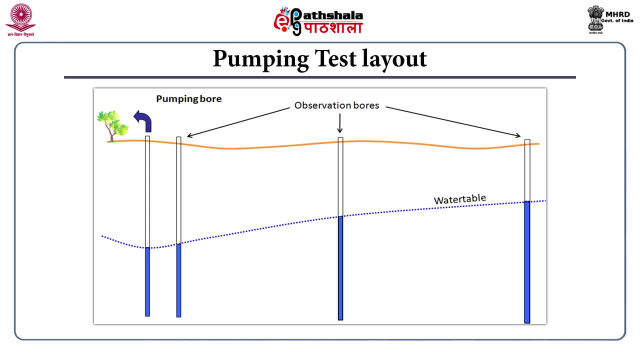 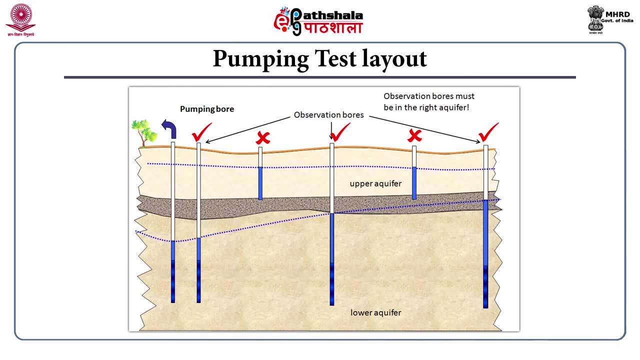 And whatever this drawdown which is going to be observed can be obtained directly from this observation wells. Now this is the another picture. this shows the drawdown and the pumping well network. One should be very careful when doing this pumping test in the field. So all 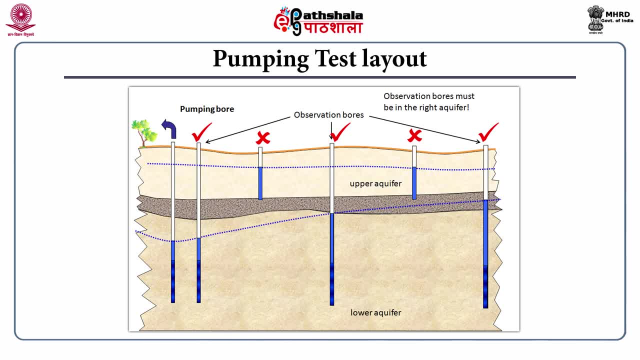 these pumping well and the nearby observation well must have the same type of the same type of the aquifer. One cannot consider the unconfined aquifer with the confined type of the pumping well, confined type of the aquifer for doing this pumping test Here, all these observation well, 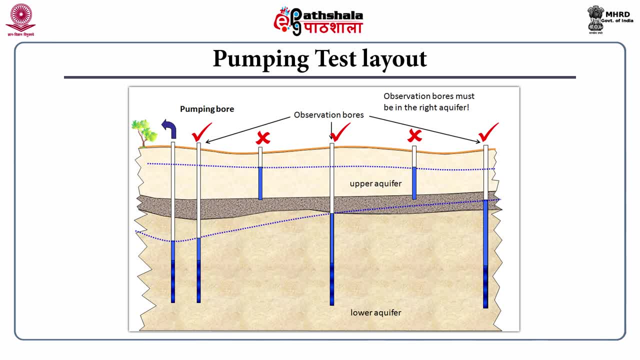 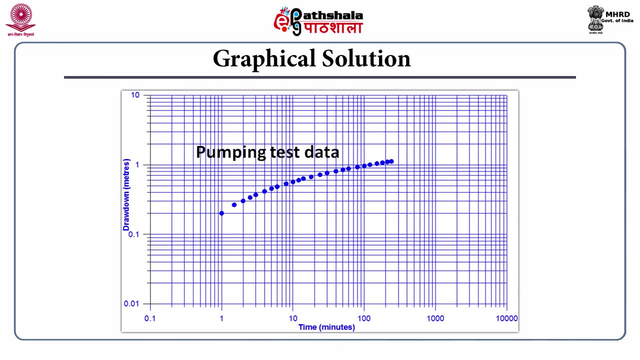 as well as pumping test should be there either in the confined aquifer or in the unconfined aquifer for characterizing that respective aquifer media. Now this is a example of the the test data, pumping test data. So in the field we can. 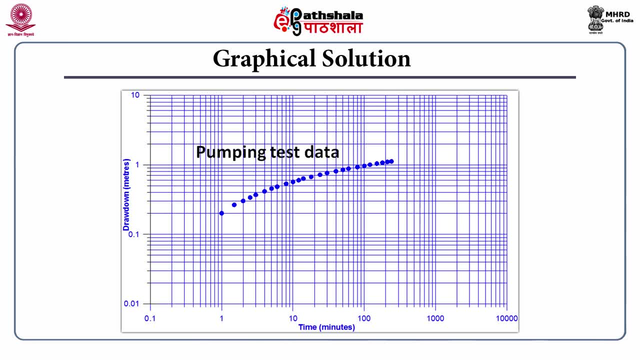 indeed can observe the time of the pumping and also we can observe the drawdown nearby to the pumping well. So drawdown is there on the y-axis and the time is denoted on the x-axis and the both are the axis on the semi log paper on the log-log scale. So that is. 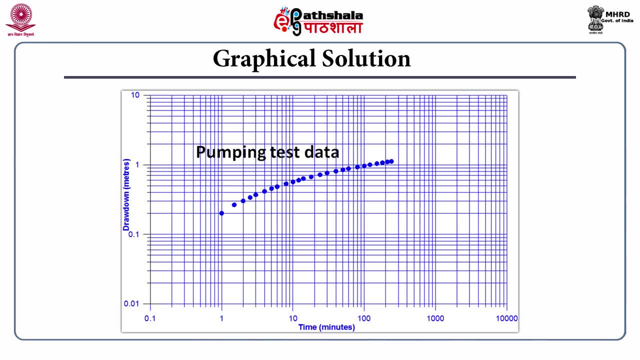 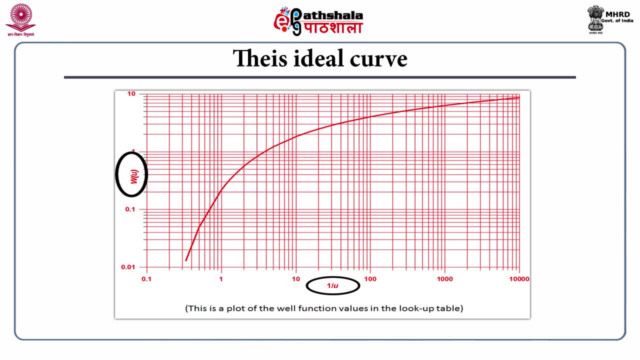 why it is known as the test data, pumping test data on a log-log, logarithmic paper. Now this well function W? u and the evaluation auxiliary function: u. that is the data curve, so the type curve. So data curve is the curve which we obtained from the field and the type curve that is already available. that is the 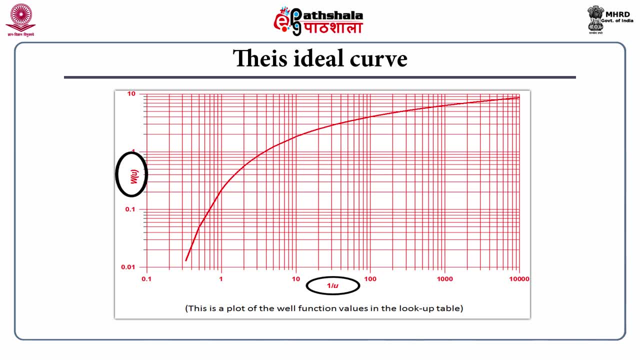 relationship between the valve function and the auxiliary function. Here it is: the valve function is there on the y axis and the auxiliary function, that is, the inversion of the auxiliary function 1 upon u, is on x axis. Now, by interpolating all these type curve, 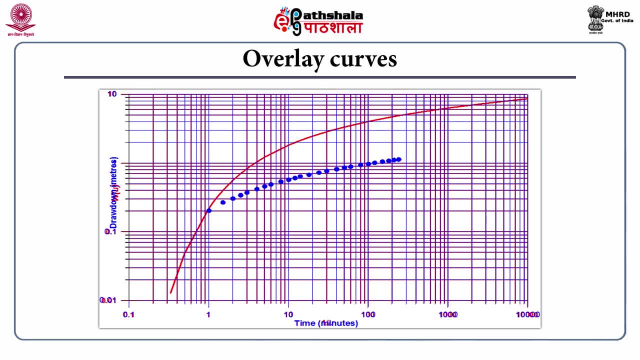 and the data curve we can obtain the overlay these two curves. So this solid line z in color shows the type curve and the blue dots are the data curve which has been obtained from the field. So by overlay of these two curves we found out a common point where these 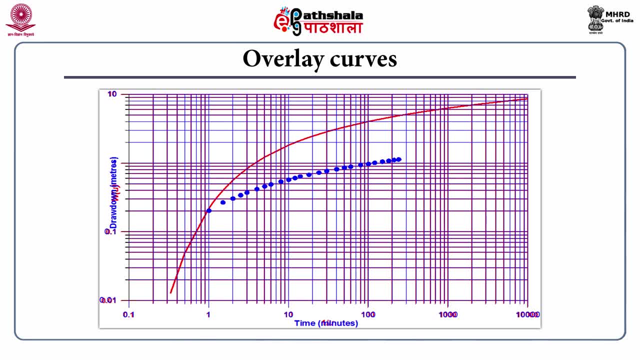 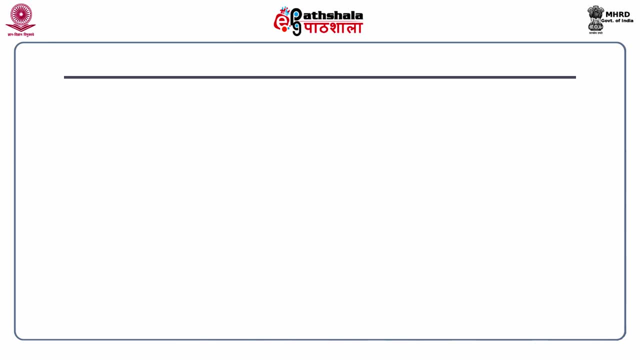 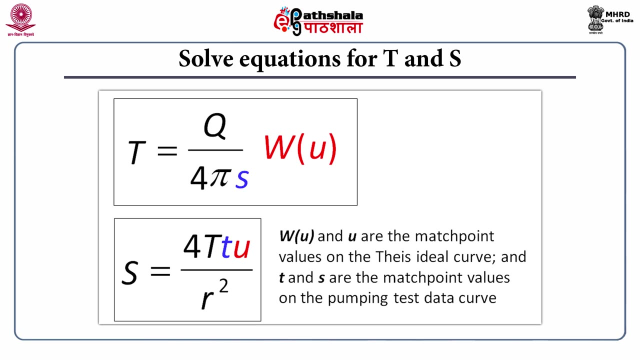 two curves are matching well and corresponding to this matching point. we obtain the data curve parameters like valve function, auxiliary function, from the data curve and the type curve. All these value corresponding to this point are substituted in this equation. The first one is: t is going to be equal to q upon 4 pi s into w? u. we already obtained the value. 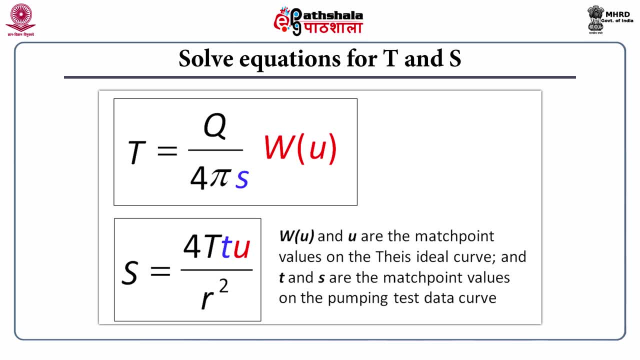 of w, u, as is obtained from the matching curve, and q is constant value, which is known to 2s and 4, pi is a constant parameter. So we can obtain the transmissivity from this equation. Once we obtain the transmissivity, we can substitute this transmissivity to this another equation. 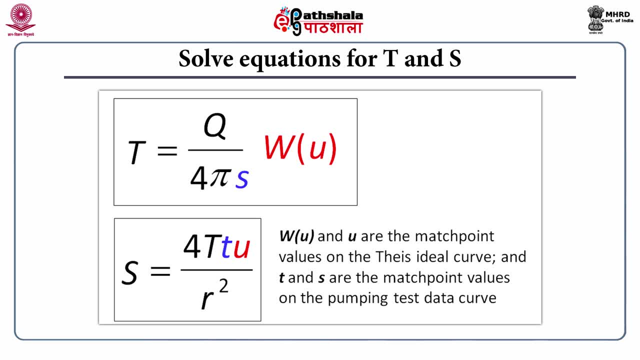 and we can get the value of storage coefficient, capital S. So this is the method that how one can get the value crucial parameter S and T with in-situ, using some pumping test data, and which are very useful especially for characterizing the subsurface system. 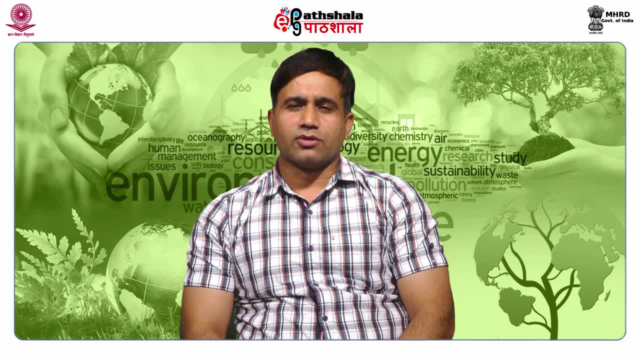 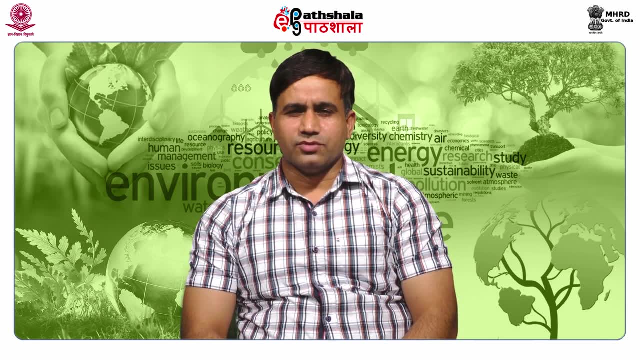 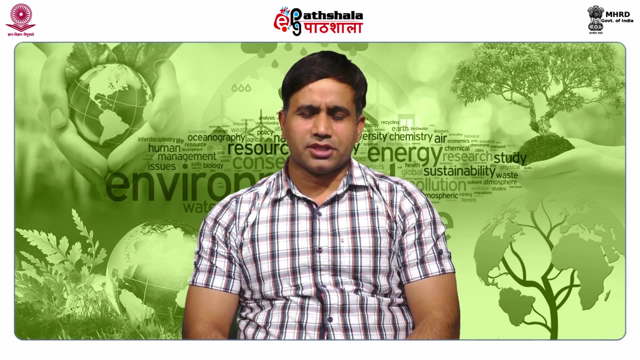 So in this module, module number 3, groundwater hydrology, we discuss about this, the main governing equations like Darcy's equation, which is the main equation for developing the groundwater flow equation. So we explained the how the Darcy's equation can be derived, where we 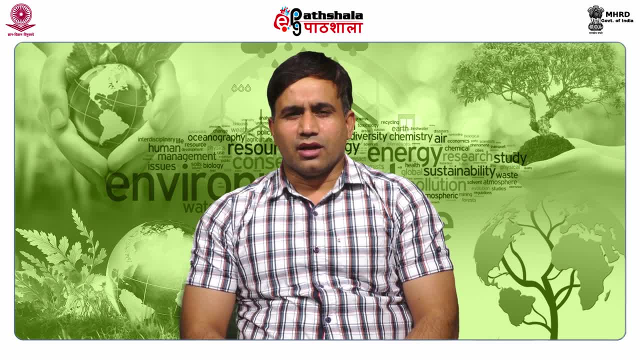 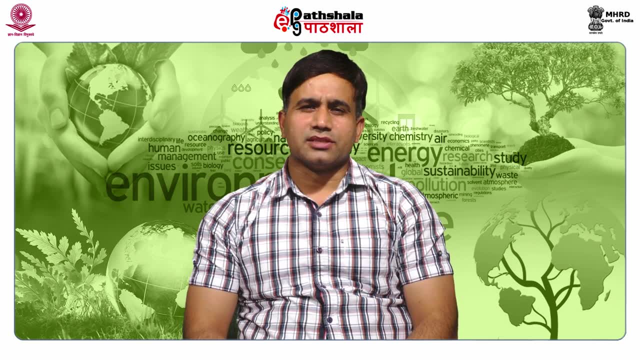 can apply the Darcy's equation with its pros and cons. This Darcy's equation can be integrated with the mass balance or the continuity equation for obtaining a general groundwater flow equation for any type of the confined or unconfined aquifers flow. 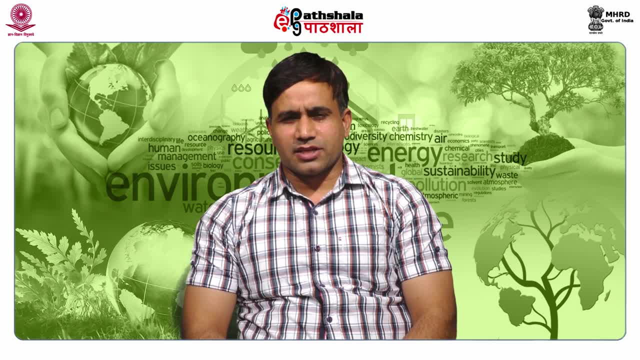 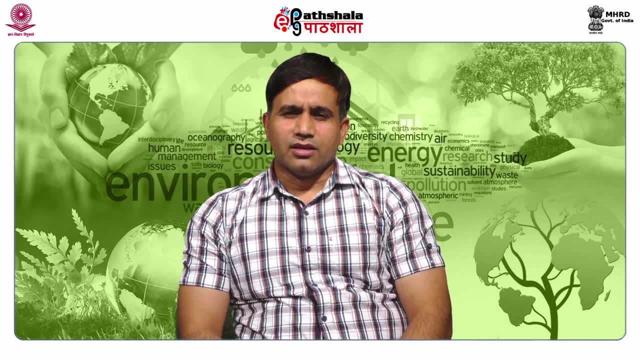 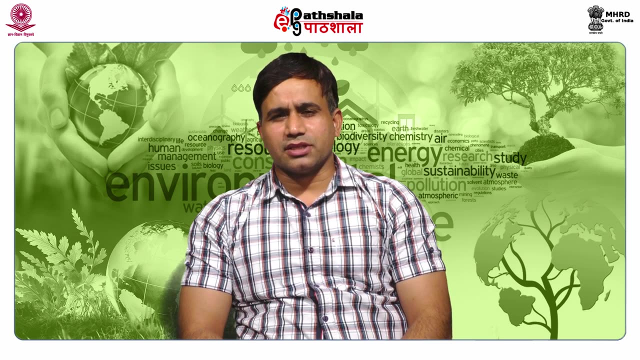 The the most you know useful equation like Laplace equation, that is for homogeneous and isotropic type of the media, can also be obtained from the Darcy's and continuity equation. Now, later on, we have also discussed about the different methods, ah before, the measuring of the hydraulic conductivity in laboratory as well as in the field. We have also discussed